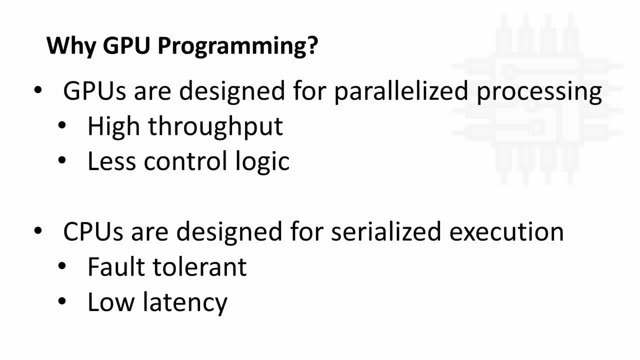 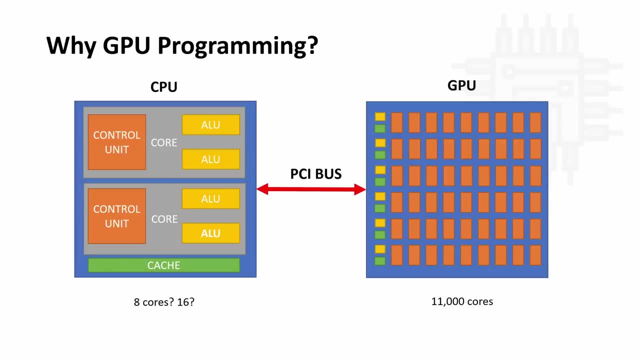 your computer to do different things. So why would we do GPU programming right? So GPUs are able to do extremely high throughput paralyzed processing. This is in comparison to your CPU, which is for serialized execution in a low latency, fault tolerant kind of way. And the reason this happens. 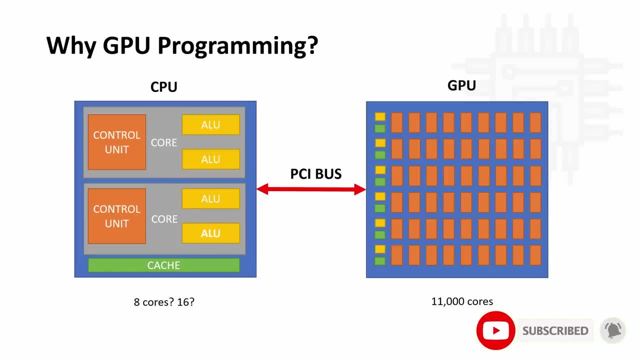 is because of the way that the CPU and GPU are designed. If you look here on the left, you have a CPU and it has maybe 8 to 16 cores, and a core consists of a control unit and an ALU right- The. 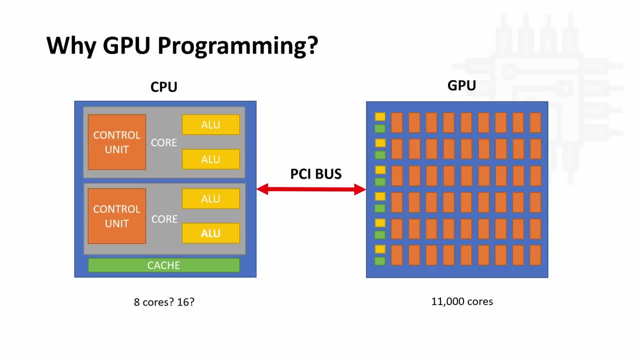 control unit does the logic control and the ALU does the math, and it has cache where it can very quickly look up memory and data as it needs. It's meant to be serialized and very fault tolerant. A GPU is designed for serialized execution in a low latency, fault tolerant kind of way, And the 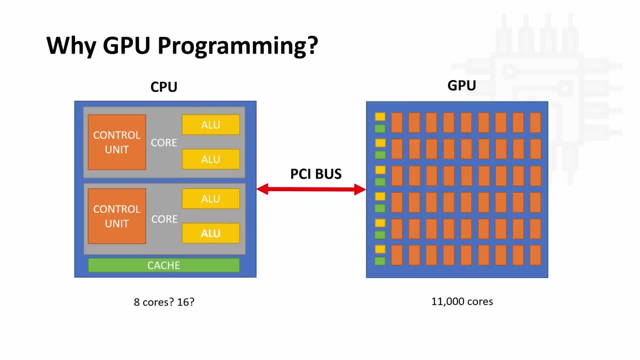 GPU, on the other hand, is meant to do things extremely fast and extremely paralyzed. They're designed with parallelization in mind And, that being said, the modern GPU- I think the 3090- has 11,000 cores, right. So if you are able to do data processing in a parallelized way, you want to be. 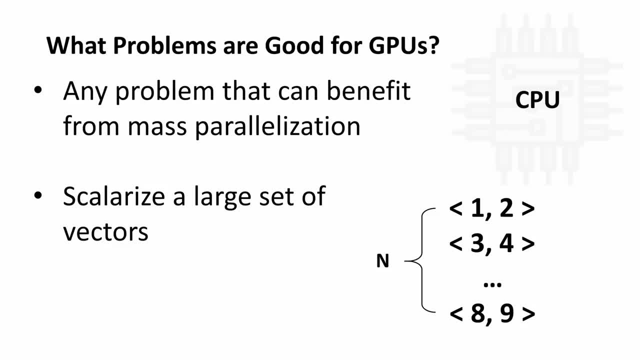 using a GPU and you'll get way faster results out of it. So, with that being said, what problems are good for a GPU? Like I said before, any problem that can benefit from mass parallelization is good for a GPU. So, for example, the common example used in talking about CUDA core programming is: scalarize a. 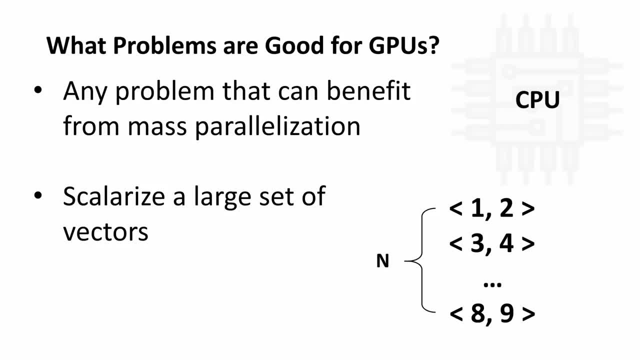 large set of vectors, right? So we're going to run through this example using the CPU model. So we have the vectors over here. 1 comma 2 is our first vector, the left column is A and the middle column is B, and then the destination is going to go into C And we have up to n number of vectors. How would 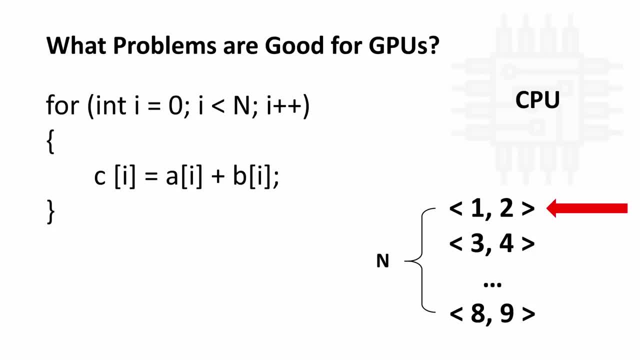 we do this on a CPU. On a CPU we would say: for int i equals zero. we would just iterate over this loop, just add them up right, Until we get to the very end. And what would actually happen in execution is we would have a very linear: lookup vector element A. lookup vector element B. add it into C. 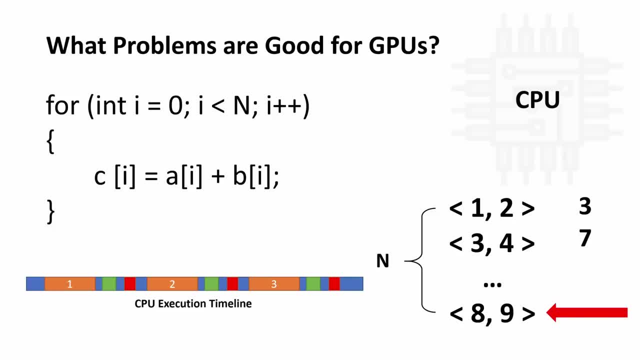 and do that for the first, second and up to nth execution. But what we actually over time get is we incur a cost in looking up and running the actual program that has to do this data lookup and mathematics, And over time it becomes less efficient to do this serialized as opposed to. 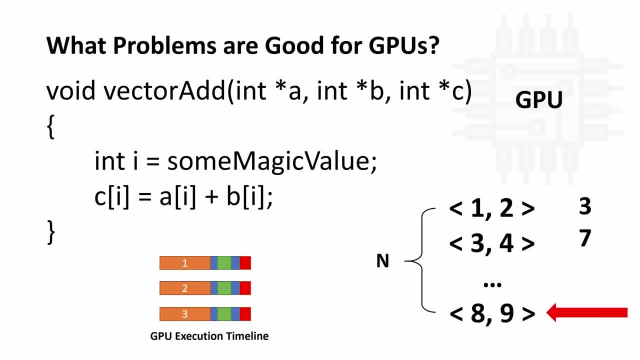 using multiple cores, And that's what we're going to do. So what we're going to do is we're going to create a function that is meant to be used in a parallelized fashion, And we would assign that function an index for every vector that we have, And we'll figure out where that index comes from. 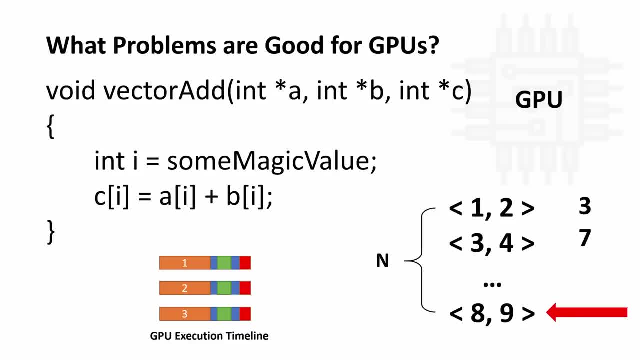 in a second. It's a pretty cool way that the CUDA framework set this up, But basically we would create this function and we would execute this function in parallel for every vector And again we're going to use the index to index into our vectors would come from the CUDA framework And 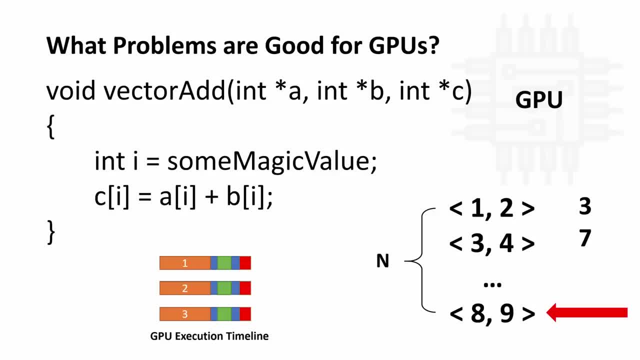 then, as you can see here, our execution timeline, right how long it takes to do this- gets cut by- in this case three. your gains would go up per the size of your n, right? So if your n is serialized out to 1024 elements, if you could do this in complete, perfect parallelization, so 1024. 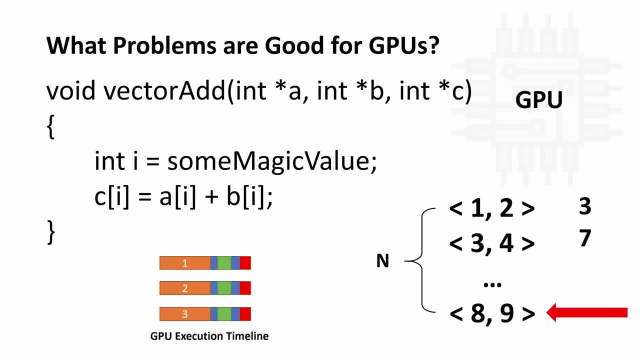 cores, you would have a speedup of 1024x, right? So how do we determine where this I comes from? I know this graphic is a little bit difficult, but I'm going to show you how to do that. So I'm going to show you how to do that. So I'm going to show you how to do that. So I'm going to. 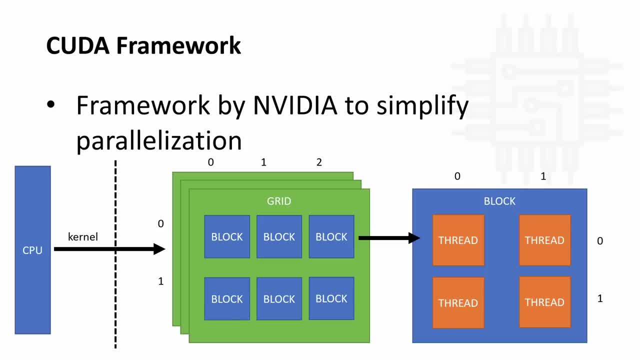 complicated, but it's actually not that bad. So the way the CUDA framework is designed, it's meant to take away the complexity of parallelization, So the abstract away from the CPU to the GPU is what's known as a kernel right, And a kernel consists of these things called grids, And then 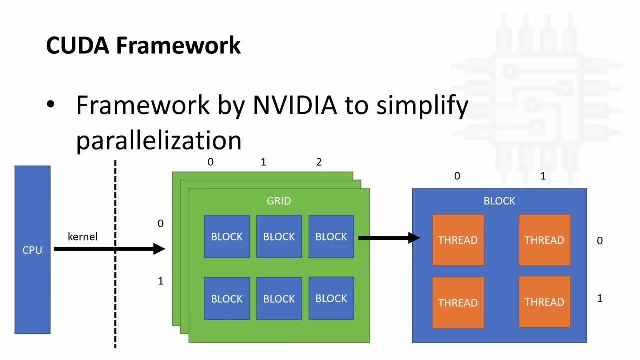 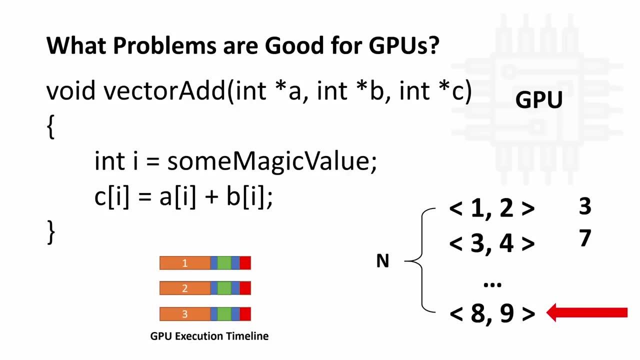 grids consist of blocks and then blocks consist of threads. And what actually happens is, when we execute a kernel, we tell the GPU how many grids and blocks and threads are going to be used to run the program. So for the case before, where we have this n value, we can tell the GPU. hey. 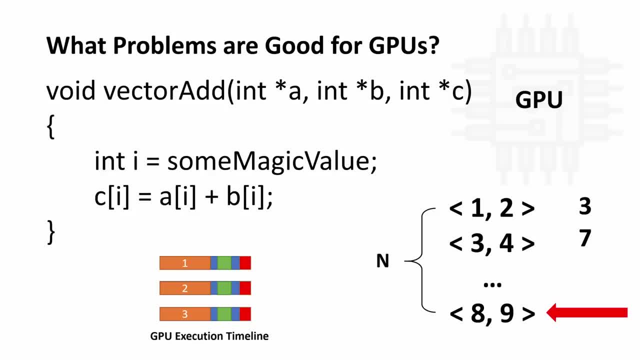 instantiate n number of blocks for this program And within that function we will actually get an index value that will represent the number of the block that we're in when this program executes. With that number we can index into the array and the block will know which index to go. 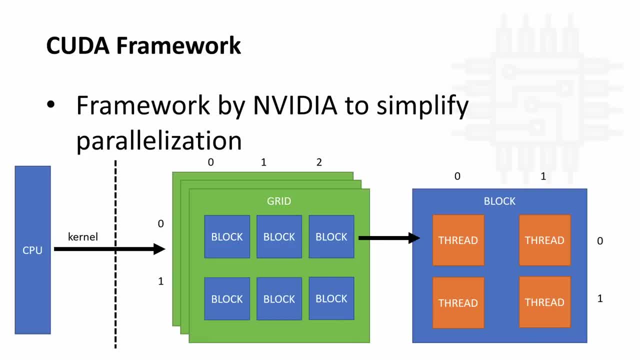 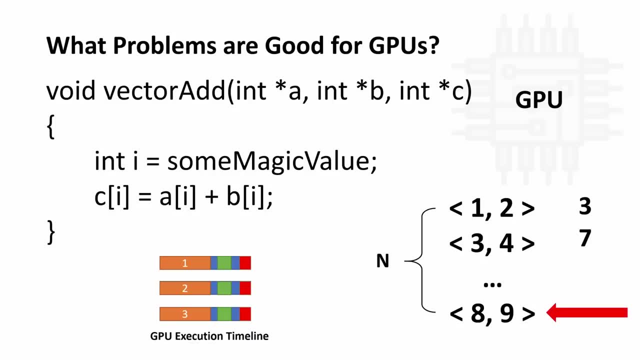 and do the math for you. So what we're going to do now is we're going to actually go into Visual Studio. I'm going to show you guys how to set up the CUDA core framework and I'm going to run you through this very example, and we're going to do it in a way where NVIDIA parallelizes the problem. 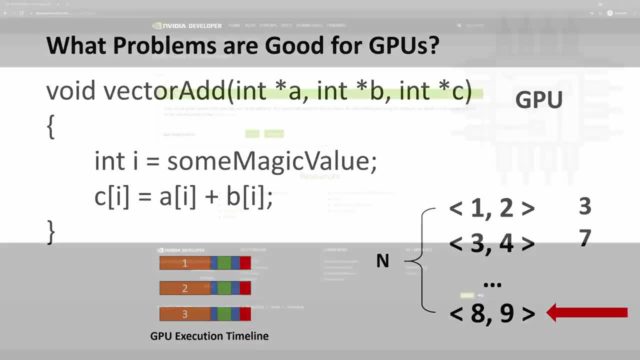 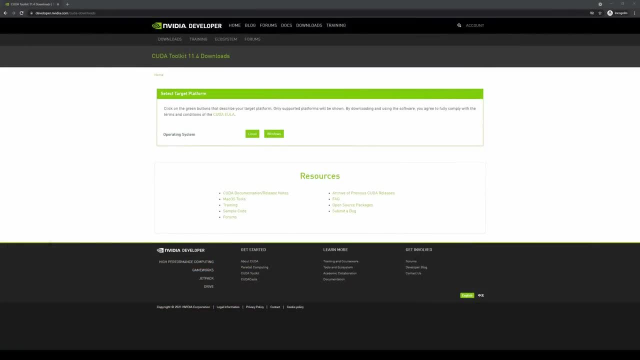 for us and does it way faster than a CPU could. Let's get into it right now. Okay, so I'm going to assume that you guys already have Visual Studio 19 installed. If you don't go ahead, pause the video. also like the video and install Visual Studio 2019.. Then what we'll do is we'll go to 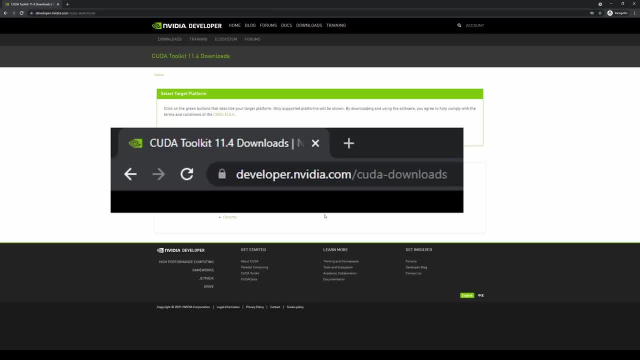 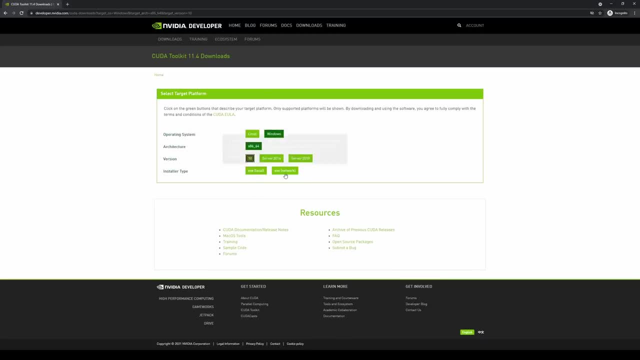 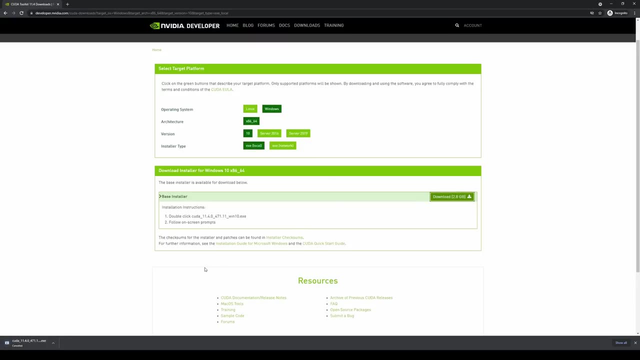 developernvidiacom slash CUDA downloads and then you just download whatever OS you have. So I have Windows x86-64, and I have Windows 10, and I would like the local version. And you go ahead and hit download and I'm going to cancel this because I already have it Once that executable gets. 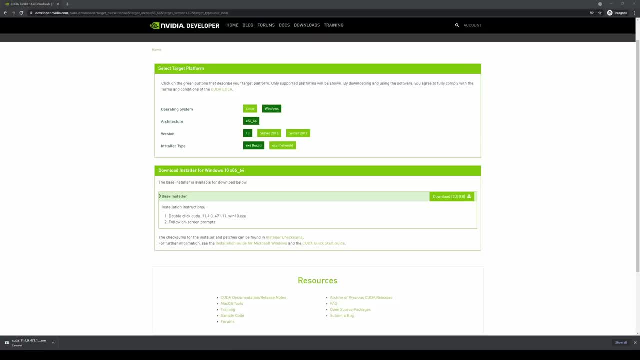 downloaded. you just go ahead and run it and I'll make sure I show you guys how that works. real quick, Let me pull it up. Okay, great, We have the installer right there. Boom, It's going to go ahead and run and it should give you the option to just do a full install. I'm not going to walk you. 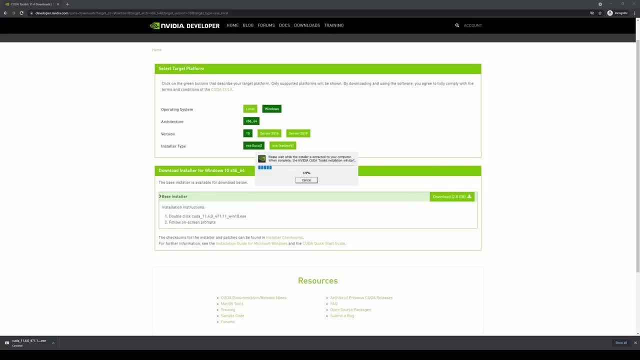 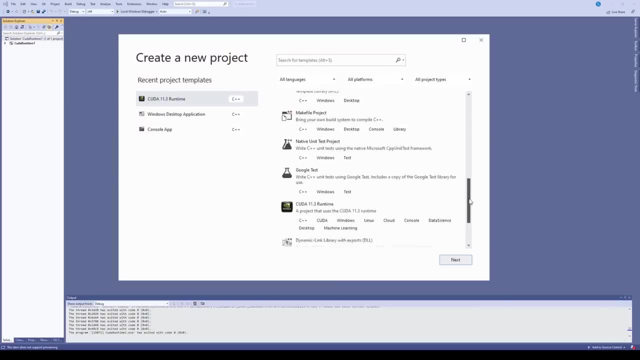 through how to do the install. I'm sure you guys can figure that out, but it's very painless. Once you get that thing installed you should be able to just open up Visual Studio and then that new project. you should have the option way at the bottom to do a CUDA 11.3 runtime project. Hit next. 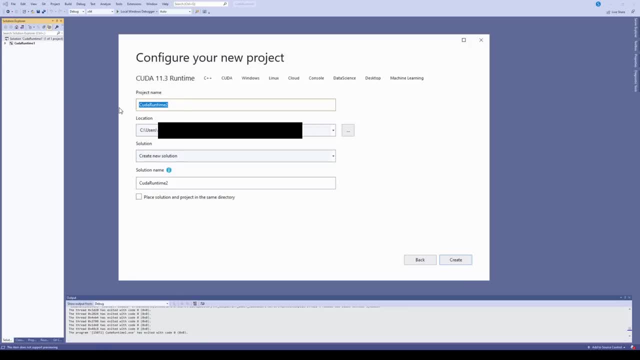 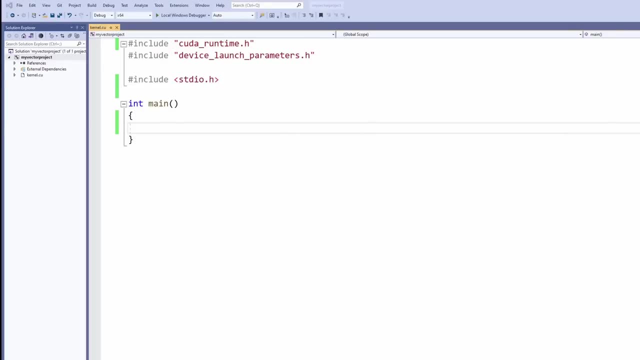 a few times: blah blah, blah blah. We'll do my vector project. That will actually give you a lot of options. I'm going to go ahead and open that project and I delete all of it, except for the include lines for the CUDA runtime header files- obviously standard IO, and then I leave my blank. 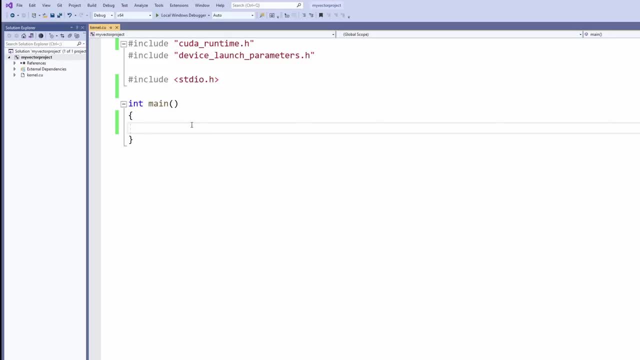 main function, right? So once we have that, we need to start writing some code. So, to go back to our example, we're going to create three arrays to represent our vectors. So one, two, three is our A, and remember that's the left-hand column of those arrays or of those vectors, rather and 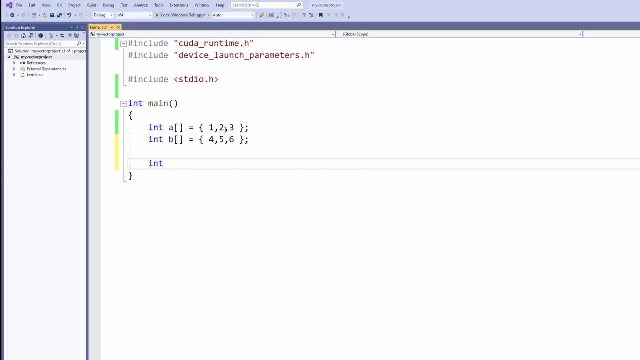 then we want to have our destination array and that's going to be of size, size of A divided by size of int, and we'll set it all to zero. Okay, great. So now I'm just going to write the CPU example, which is really simple, right, For I equals zero, I less than size of C over size of. 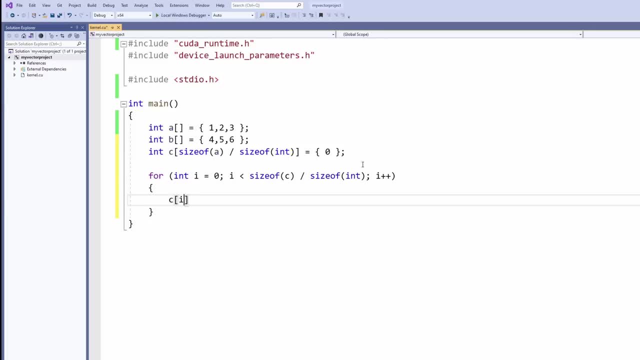 int. I plus plus C of I equals A of I plus B of I, And we'll say return and we're going to want to break right here to prove that C actually got set. So it should be right: five, seven, nine, We'll run. 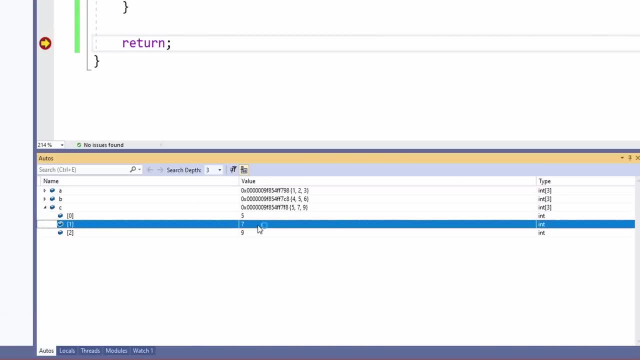 that real quick. Yep, let me see here We got five. I'll zoom in for you guys. Actually it's pretty small: Five, seven and nine in our vector Right, very, very cool. Okay, well, that's. 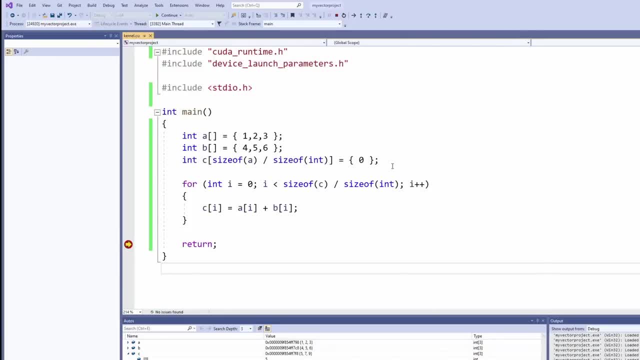 boring. That's the CPU example. We want to use the CPU example and we want to use the CPU example to do this right. How do we do that? There's a couple things we have to do right. So first, 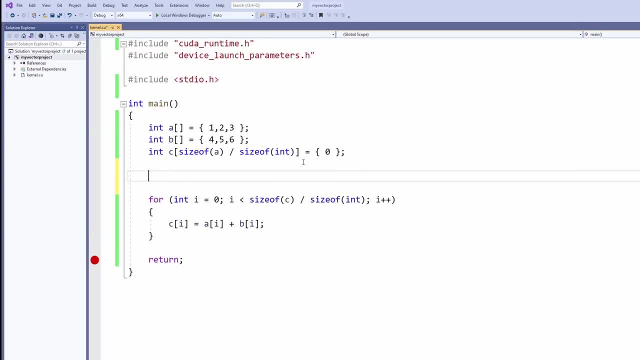 we need to have a pointer that points into memory that is controlled by the GPU. So we're going to have int star. CUDA A equals zero. This is going to be a pointer to the GPU's memory. We're going to do that actually three times and that'll be CUDA B and CUDA C. 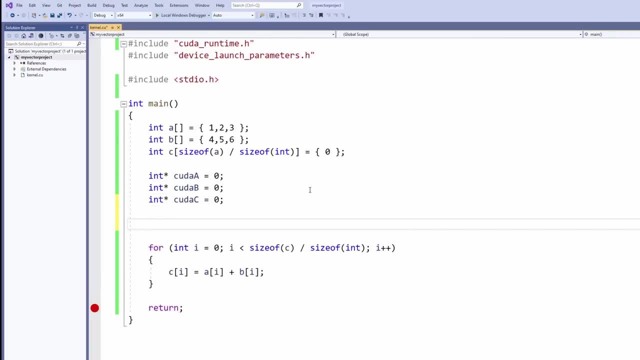 What we want to do is we're going to do a pointer to the GPU's memory. So we're going to do a pointer to the GPU's memory. So what we want to do is we want to actually allocate memory in the GPU to copy our data out to The way we do. that is, with CUDA Malik, And CUDA Malik takes a pointer. 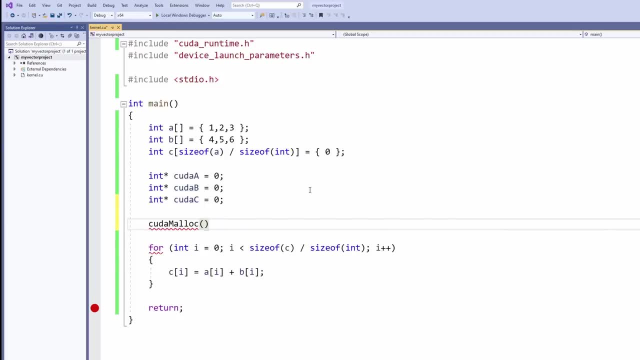 pointer. So we're going to actually overwrite CUDA A on the stack with this value, right? So it's going to be the address of CUDA A. And how much do we allocate? We're going to allocate size of A bytes, And that's correct, because this is the size of A And we can just copy this and do it. 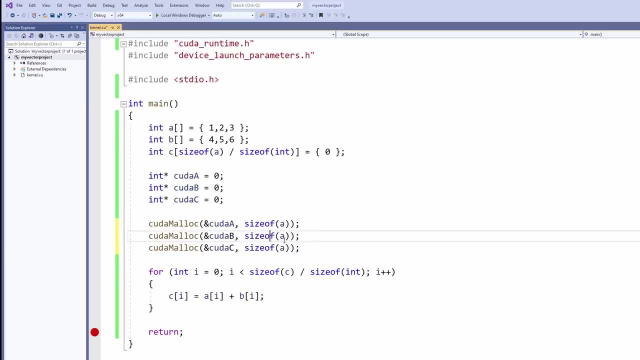 three times: Allocate CUDA, B, CUDA, C, CUDA, and then A, B and C. Okay, great. So if this all happens correctly, which we should check for? return values? but today we're being bad programmers. we should get pointers into the GPU that have enough room to hold all of our vectors. Okay, 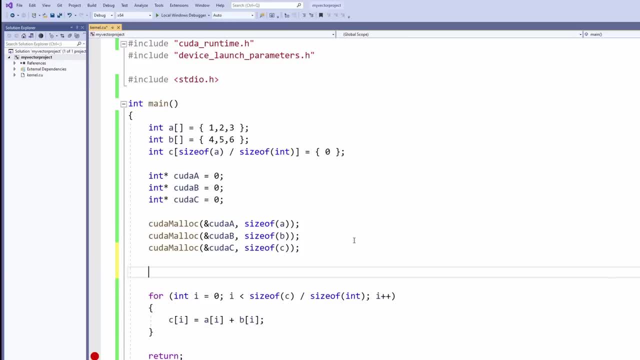 so now that we have all the room to hold our vectors, we need to put the vectors into the GPU for processing, right. So we use CUDA mem copy to do this, and the destination is going to be CUDA A, The source is going to be from A and the count is the size of A. This is your standard mem copy. 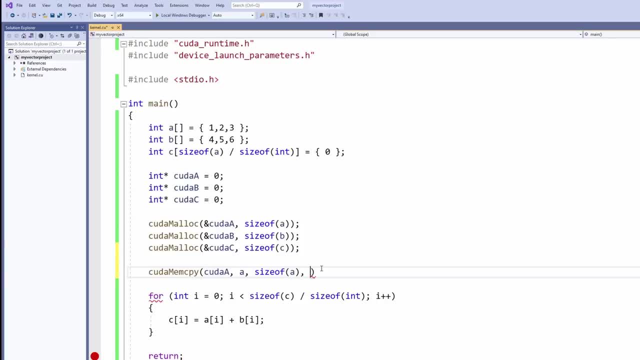 right. You have destination, source and size. The final thing you have to do is you have to actually tell the CUDA framework what direction is the data going? Is it going from the host to the device or the device to the host? So the host, in this case the CPU, the device the GPU, And in 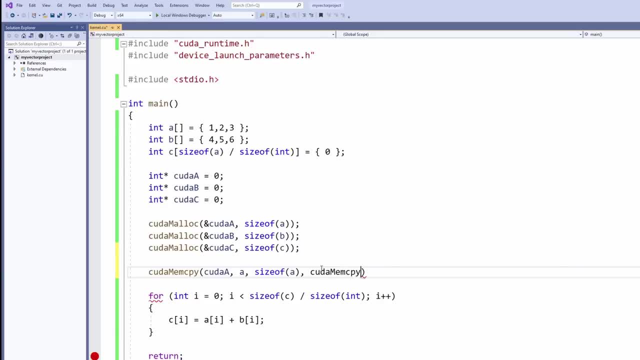 this case we are going from CUDA, mem, copy, host to device And we can again copy this three times: Boom, boom, boom, CUDA B, CUDA C, B, C, B and C. Okay, and we're going to start commenting to make this a little. 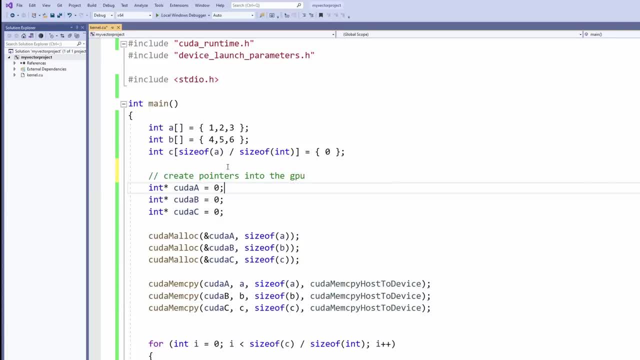 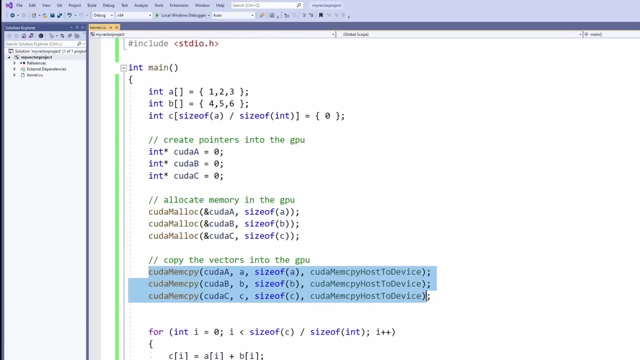 easier. So create pointers into the GPU, allocate memory in the GPU and then copy the vectors into the GPU. Okay, pretty straightforward, right? Create these pointers, malloc memory to them and mem copy into them. Great, And we're going to get rid of our CPU example because, again, 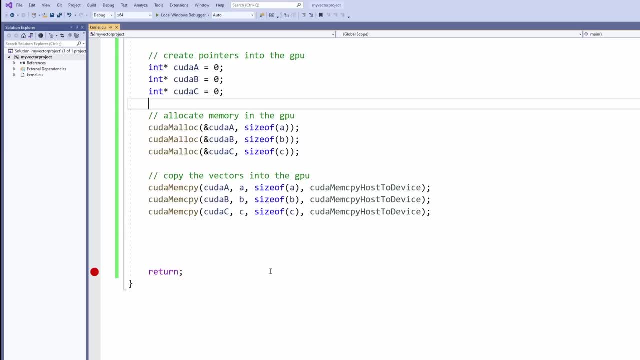 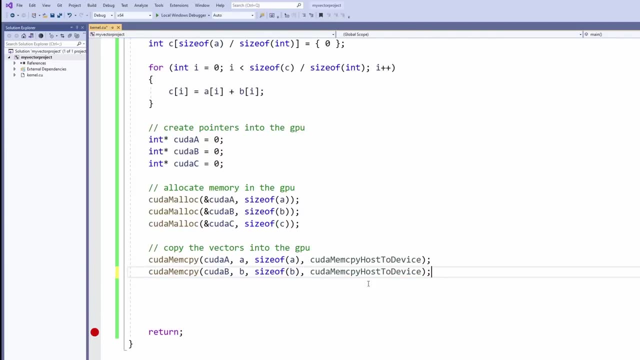 that's hyper boring. No one cares about CPU. Great, So now we have our memory put into. actually, we can just skip this line because it's zero at this point, So we don't have to do that. Now we want to run our code that adds these: 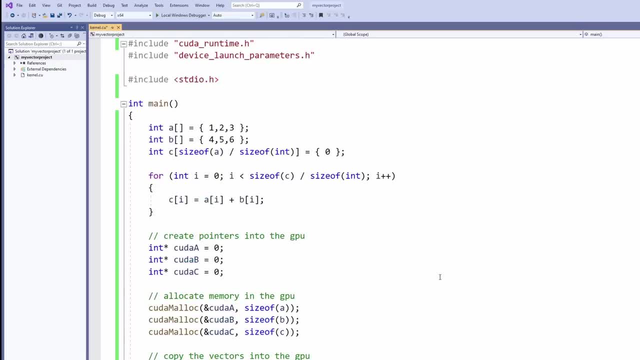 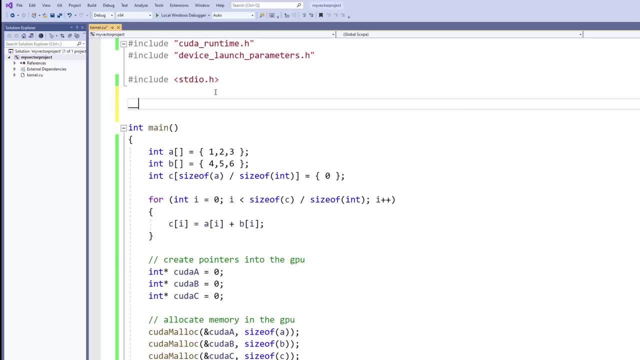 vectors together. Okay, so how do we do that? Well, first we have to write our program that gets ran in the GPU, or write our function. So the way you do that is what's called a double, double global. Double, double global tells the compiler that this is going to be a function that. 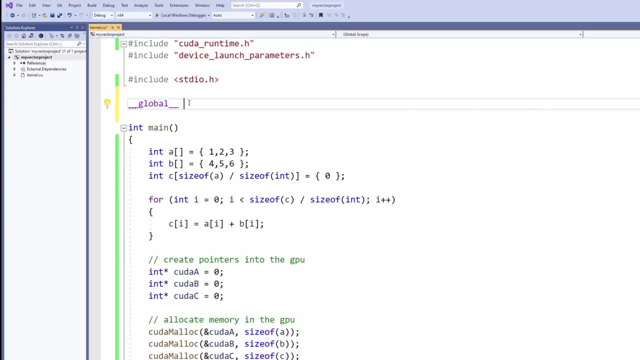 runs in the GPU, So it prepares it that way and it creates the memory maps so that the GPU knows how to pick it up. Okay, so then we say void, because we don't want it to return anything. And then we say vector add And it's going to take three parameters- A, B and C- And note these: 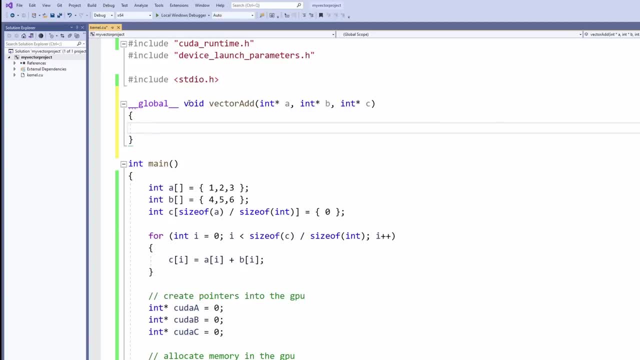 are all pointers right, Because we're giving a function that is able to be parallelized to the GPU, And then the GPU is going to handle it using the CUDA block grid thread framework, right? And then what we're going to do is we need 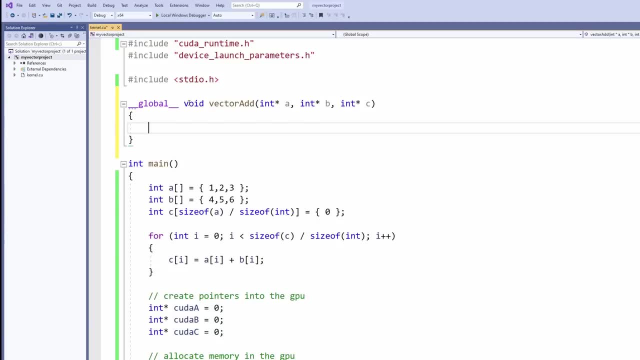 to access the elements based on the index of the thread that we are, And the way that works is we say that int i, which is our index we're going to use to index into the arrays, is equal to thread idxx. So what this means is that we are going to create a list of threads. 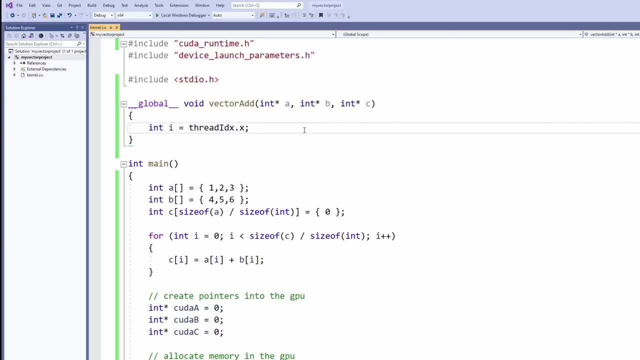 and this will get called on: every vector in the list. This x value is going to represent the number of the vectors that are going to be called on- every vector in the list- And we're going to use that to index into these arrays and add them up. 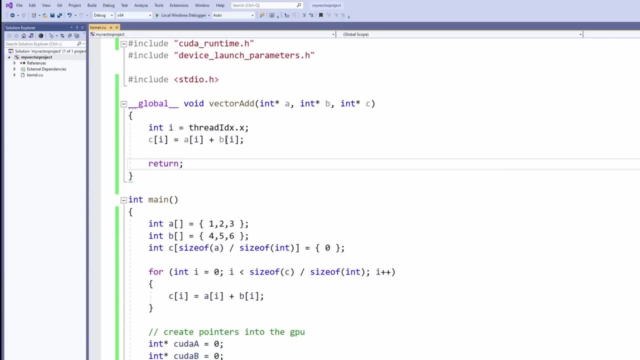 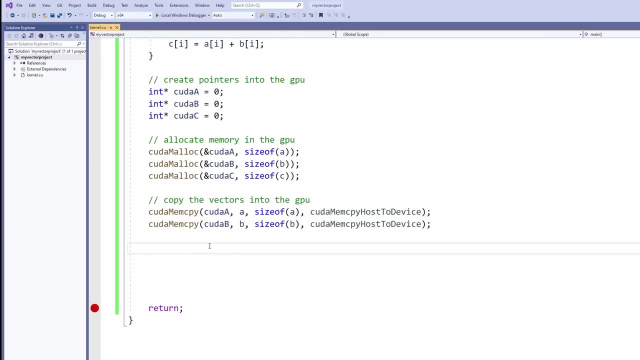 Boom, there we go And then return. but it's a void, so it'll automatically return. Okay, great. So now we need to instantiate this. We need to run this right. How do we do that? The way we do it is we say the name of our function, vector add, but then we have to add: 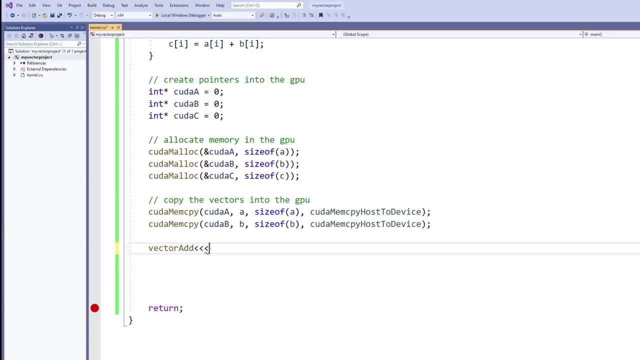 the special syntax, which is one, two, three carets, And the syntax that we're going to use is grid size, block size. We're not actually going to leave this here, I just want to kind of explain this. So the grid size is the size of the grid, which means it is the number of blocks that we 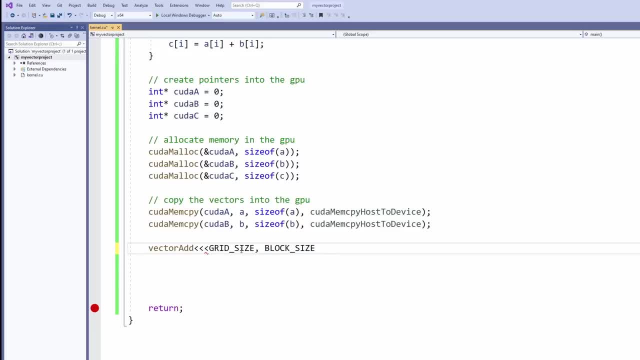 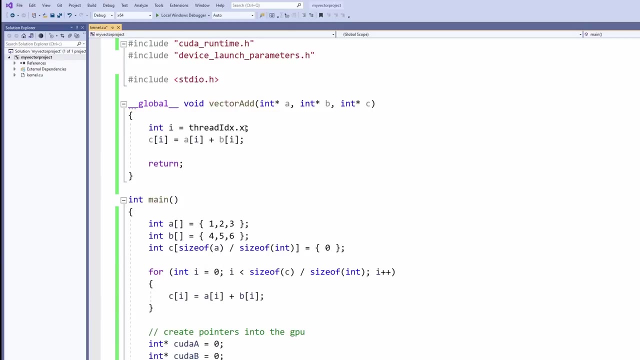 have. And then we say the block size, So per amount of blocks. in here this says how many threads exist per block. So I'm going to say we only want one block because it's not a very big program. I don't want to over parallelize it And that will actually cause issues here if I do that. 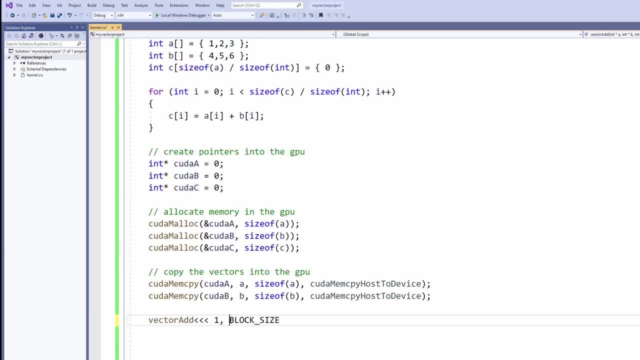 I don't want to do anything outside of one block. And then the block size is actually going to be the number of vectors. And what is the number of vectors? It's size of A over size of N. And then I call it with the parameters CUDA A, CUDA B, CUDA C. So at this point and again, 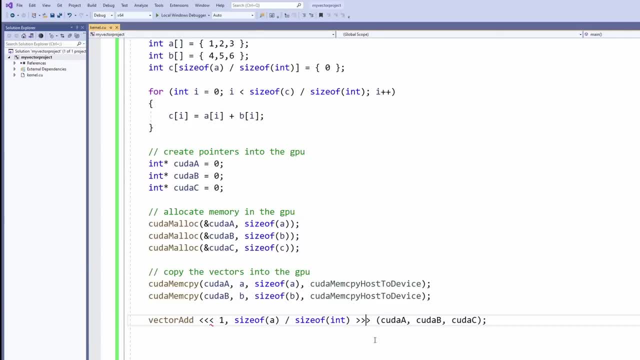 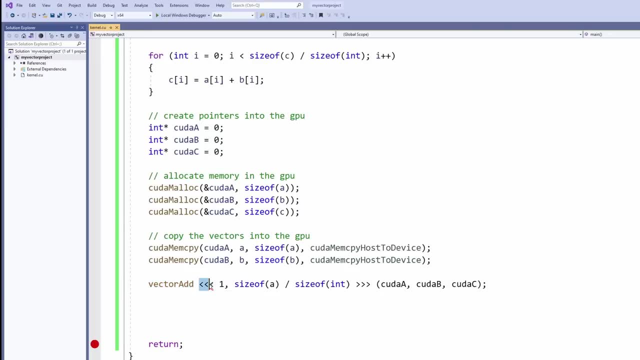 there's going to be an error here. It will actually compile. just fine, You can just ignore this. So what will happen here is the CPU will tell the GPU: hey, run this function vector, add in a CUDA kernel with a grid that has one block And that block has this many threads, and call it with: 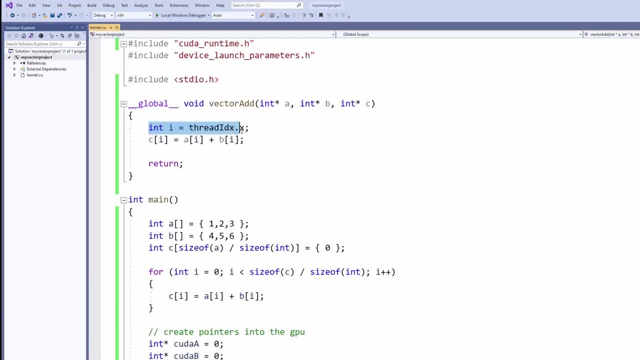 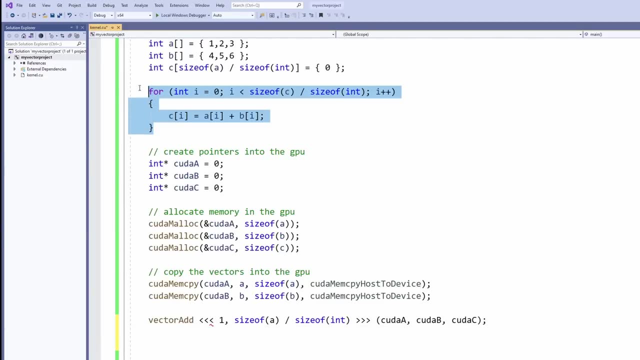 these parameters That will get ran here, And then for every thread we do our thing and we add the values together, right? And then finally, once that happens, I'm going to delete the CPU part, first because I want to confirm to you guys that you know this actually happens. So then, once we 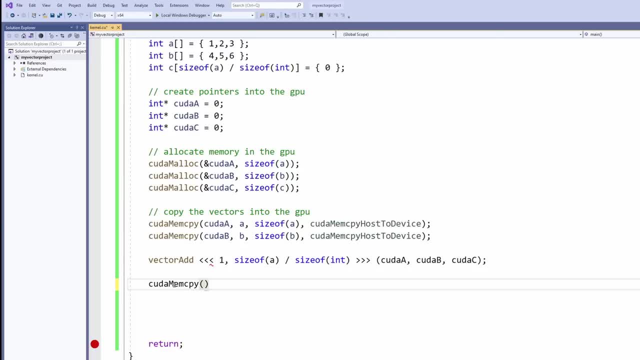 have that. we want to CUDA mem copy the result out of CUDA C. So the destination is going to be C, The source is going to be C, And then we're going to do the same thing here. We're going to do the. 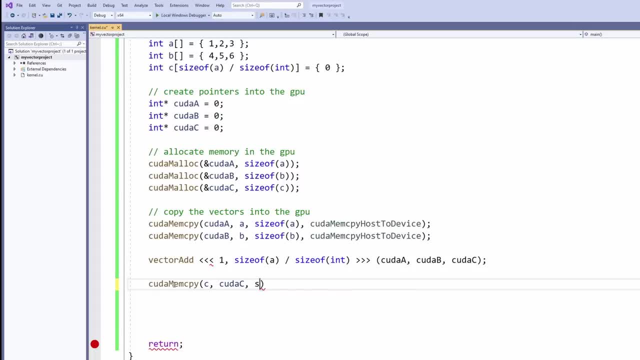 CUDA C And then the size is going to be size of C And instead of being a host to device, this is going to be a device to host. And again we're going to break right here and just prove to you guys that that happened. So we'll go ahead and run this. So we're at the return here. So here is C. 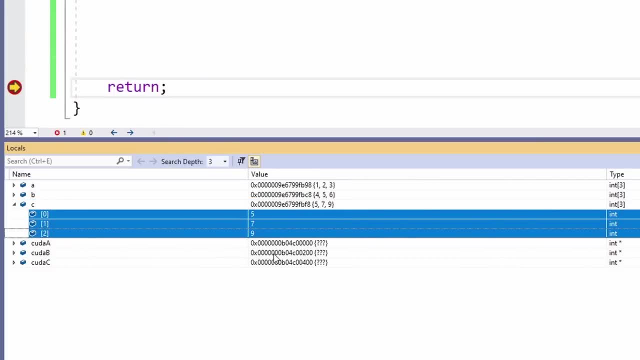 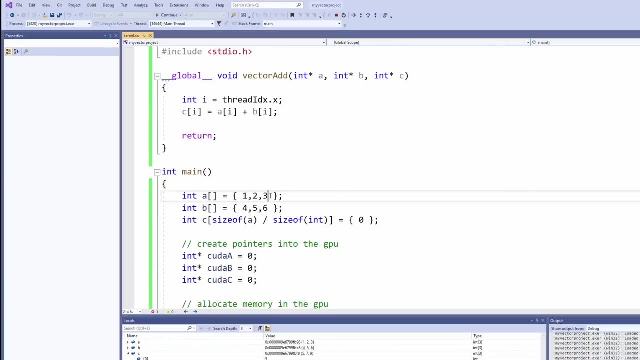 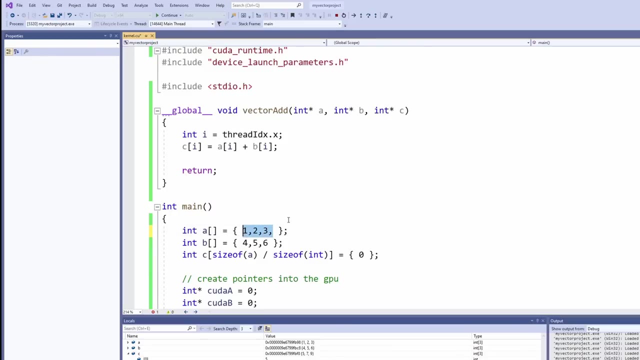 You can see that C579 got parallelized and it actually added them in the GPU and then it brought them out. So what we can do is we can actually make our vector a little bit bigger here. So I'll copy this bad boy, I'll make B the same way, And then C will grow dynamically with that. These 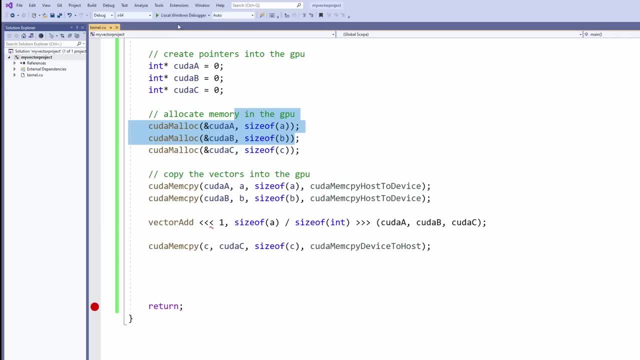 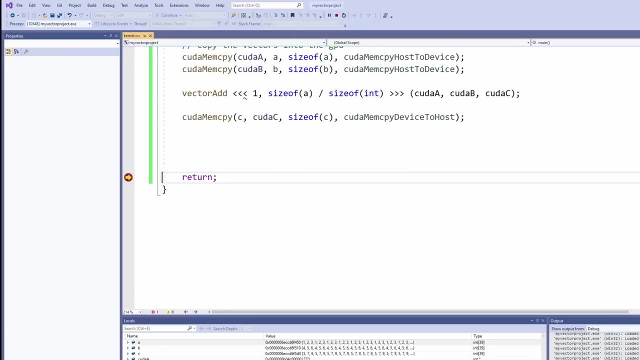 things will all be the same, Yep. So we can actually stop and run this again. I'll show you guys how it works. It should, based on this number, properly instantiate and add our vector together. Yep Boom. So you see, that would happen. So we're going to copy this bad boy And then we're going to 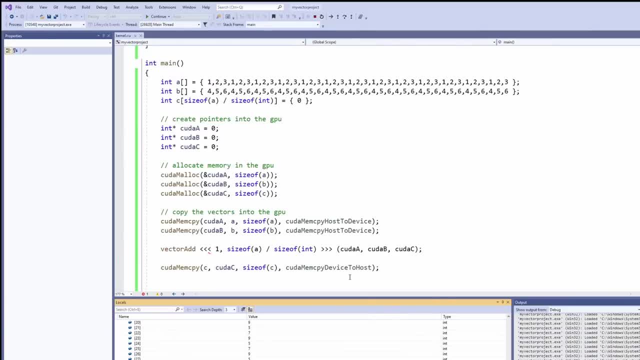 see, is it just added all these together. So again, pretty cool, right? What's happening? We're creating these vectors locally on our computer. We're creating a destination register on our computer. We're saying: these are going to be pointers into the GPU. We allocate memory in the 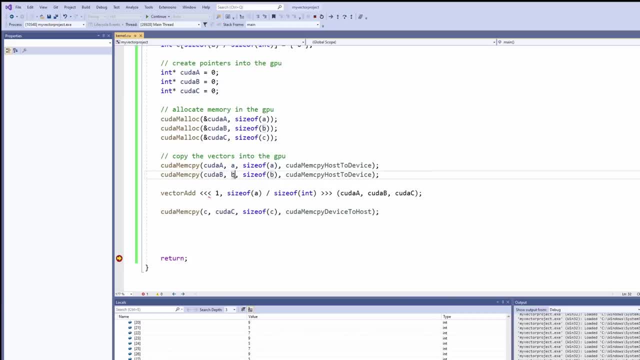 GPU and overwrite those pointers. We then mem copy from our computer to the GPU using this flag here, And then we say: run this function this many times in parallel with these parameters And then, once we've copied that memory out of the GPU, and then we display it here. Guys, I hope that was useful. I. 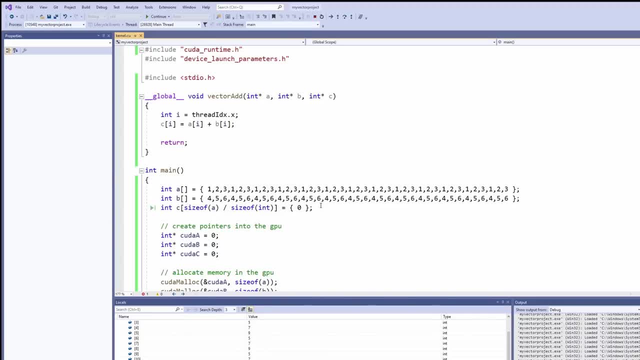 hope you guys learned something. The power of the GPU is very, very high. You just need to learn how to write a program that can parallelize in a way that can be useful when you're doing CUDA core programming. If you guys enjoyed this video, do me a favor: hit like, hit, subscribe and I'll see you. 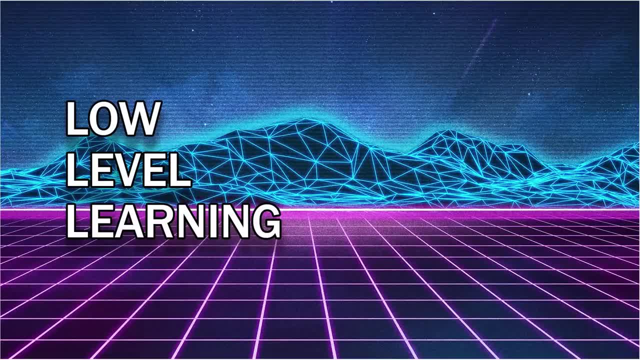 guys in the next video, Take care.